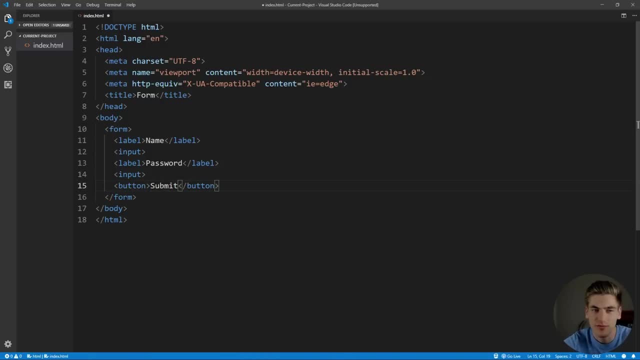 So let's just create a button here and we're just going to call this submit for the text of our button. Now to actually test this page, we can just right click and open with Live Server, which is an extension from Visual Studio Code that you can download. Once we have that opened, 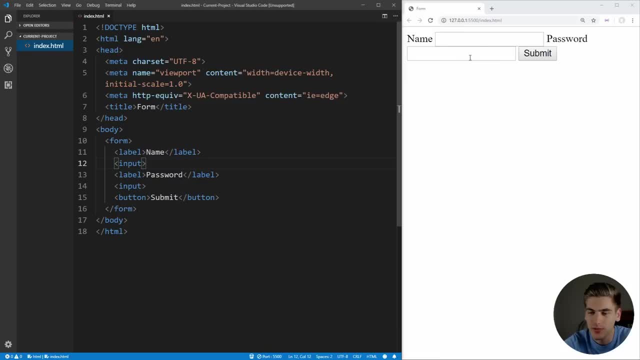 we can see over here that if we expand this a little bit, we have our name field, we have our password field and we have our submit button, And right now they're all clobbered onto the same line. so let's use some divs, which is just another basic tag which will allow us to separate these. 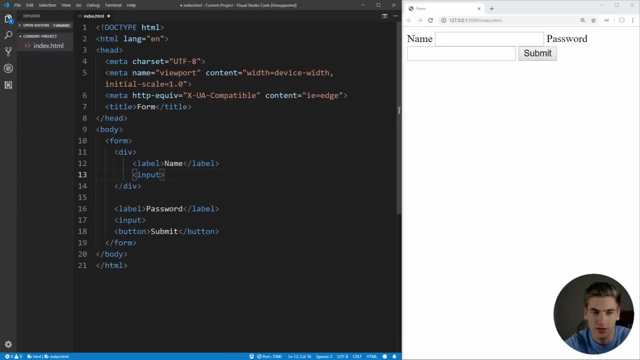 onto multiple lines. So if we put some code inside of this div, it's going to end up on the next line and we can do the exact same thing down here with our password. Let's create another div to wrap our password element in Whoops. Copy this, Paste it in there And when we save, 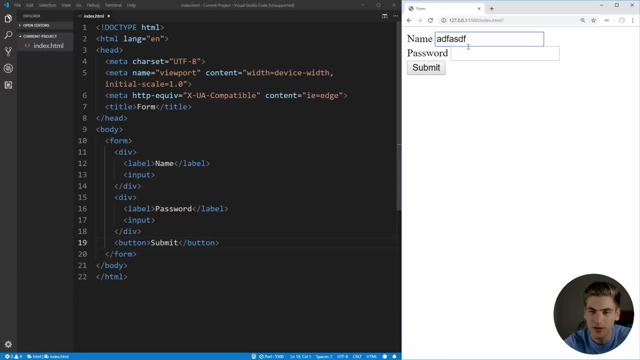 you see it populates over here on new lines. Now we can enter name information, password information and click Submit And you'll see it'll submit it to the page that we're already on. But while technically this does work, it's not at all how you want to build forms in actuality. 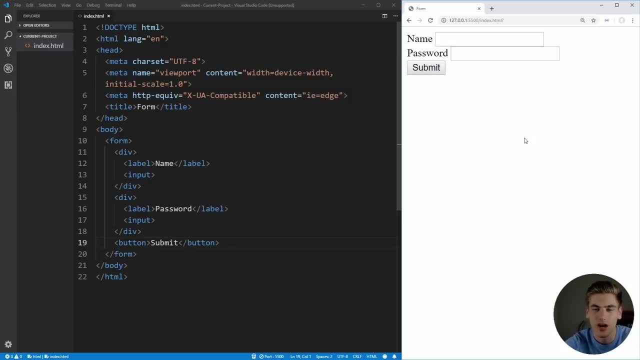 Almost always, when you build a form, you're going to want your form to be submitted somewhere other than the page that you're currently on. So in order to do that, we have a keyword here, an attribute, which is called action, And the action is going to be where your form is submitting. 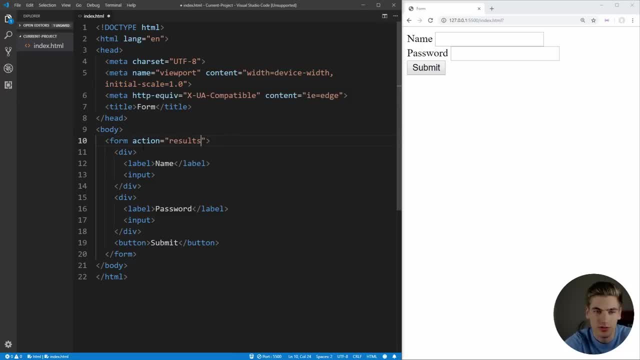 to, And in our case, we're just going to create a page here which is called resultshtml, And this is going to be where we want our form to submit to. The next thing that you almost always are going to specify on a form is going to be where you want your form to submit to. So in this case, 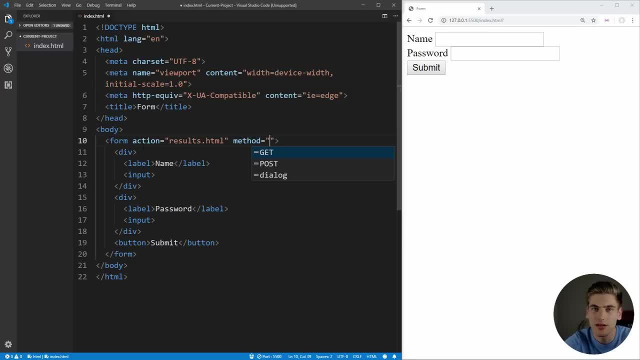 the method you want your form to use, And this is either going to be git or post. With a git request, it's going to append things to the URL and it's going to send it to another page in your site, while a post is going to be useful for when you have a server where you need to save some. 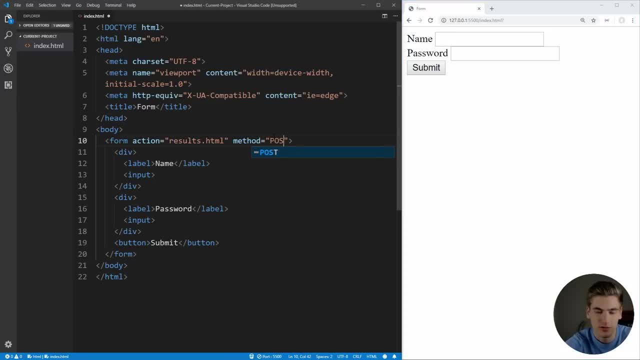 information If, for example, we were to use post here. so if we change this to post and we try to submit something, you see that we're immediately going to get an error because browsers can't render post requests, They can only render git requests and we don't have a server. 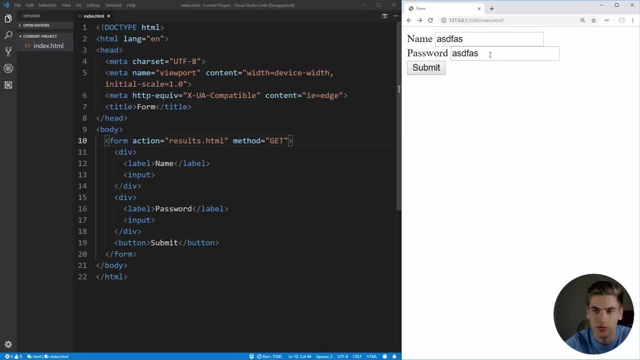 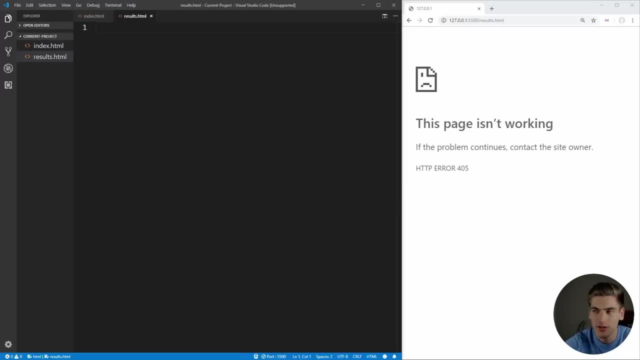 So what we need to do is we need to use a git request here instead of a post request, And now this is going to work as soon as we create our actual page. So let's create that resultshtml page, and I'm actually just going to copy over here a resultshtml page. This is a very 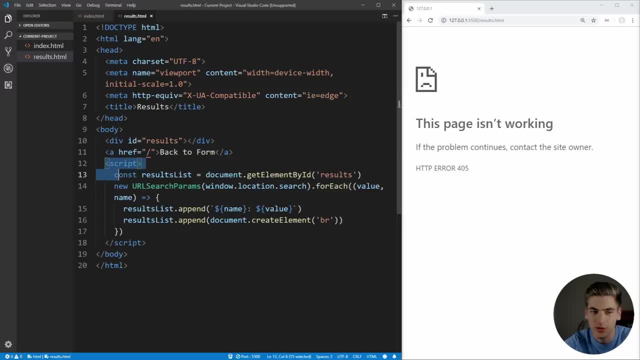 basic page. All it has is a link that goes back to our form, and it has a little bit of JavaScript which is going to render the results from our HTML form from before. So now let's go back over here, refresh our page, and we want to just make sure we click submit And you'll see that nothing is. 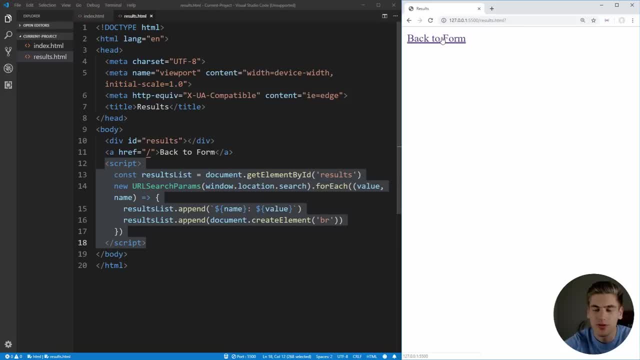 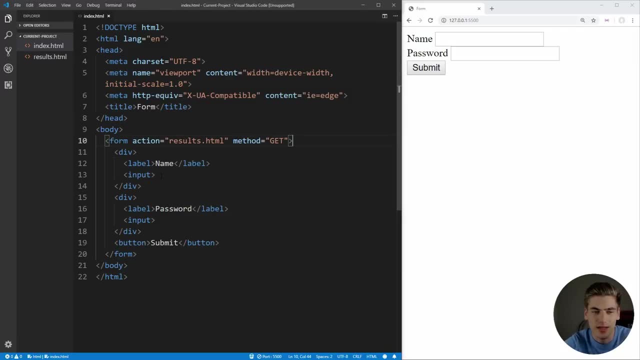 being shown up for our form fields, but we do have that button to go back, And the reason nothing is shown up for our form fields is because, in order for an input to actually show up as a form, what we need to do is we need to specify the name for that input. So let's do that now. The name here is just: 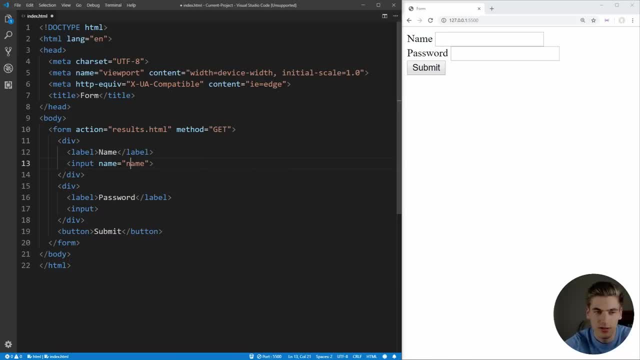 going to be name for this first one, because we just want it to be whatever we're submitting to our form. So we're going to use this as name And down here for our password, we're going to set the name of this one equal to password. Now, if we save that and come over here and we type in for 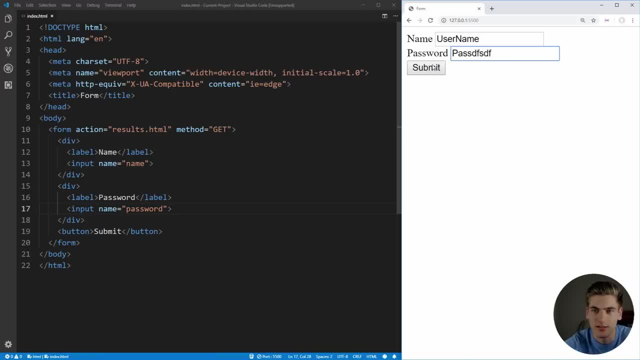 example a username and we type in a password. let's just say that's that and we click submit. you'll see name is set to username and password is set to password And if you can see in the URL, it's setting those parameters here: name equals username and password. 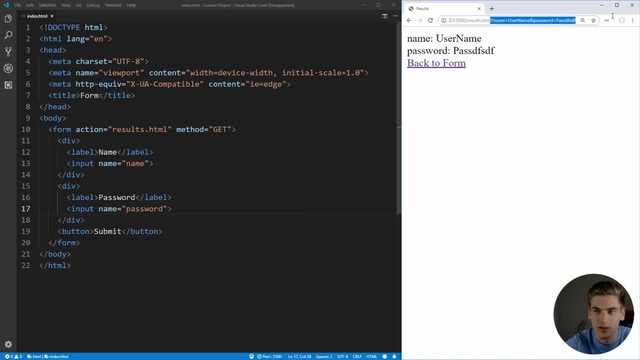 equals password, And that's what a git request does, is it sets it in the URL here, While if we did the post request here, this is actually going to set it in the body. So if we refresh this, enter in some information and click Submit Again, we're going to get that error because we don't have a server. 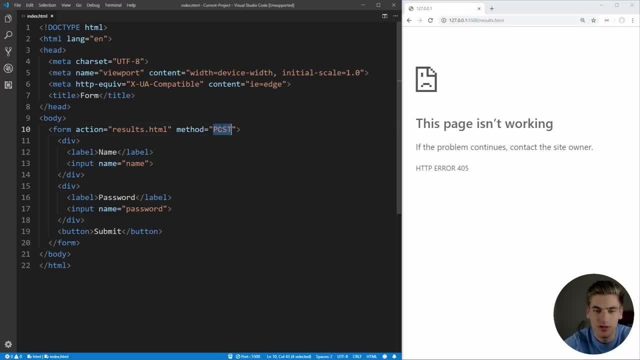 accepting any request. So you need a server if you're going to use post. So for the rest of this example, we're going to be using git for all of our different requests. So now, with that out of the way, we have our form set up properly, we have our input and we're going to go ahead and 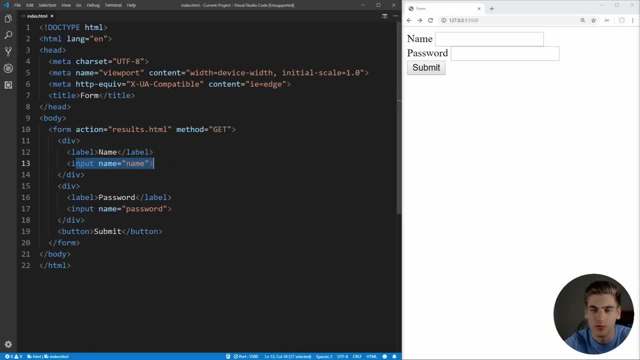 add inputs with actual names so that we can use these and render them later when we submit our form. But our labels aren't actually doing anything very useful, Because normally if you click on a label, it should actually highlight the field that it's being labeled for. This is 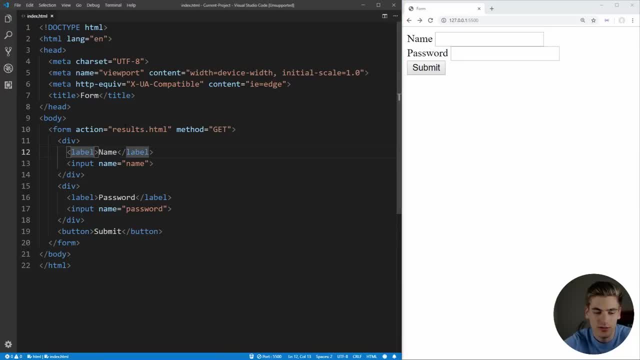 really helpful for not only users but also for screen readers. In order to do this, we just need to set a for attribute here And we set it to the ID of the element that we want to highlight whenever we click on the label. So in our case we're going to say name and then we need to give 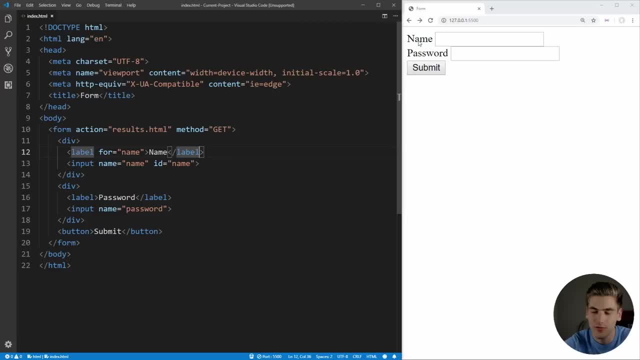 our element here, that ID which is just going to be named. Now, if we click on our label, it's actually going to highlight the input element that that label is for. Another way that you can do this is, if you don't want to have that for attribute, you can actually nest your element. 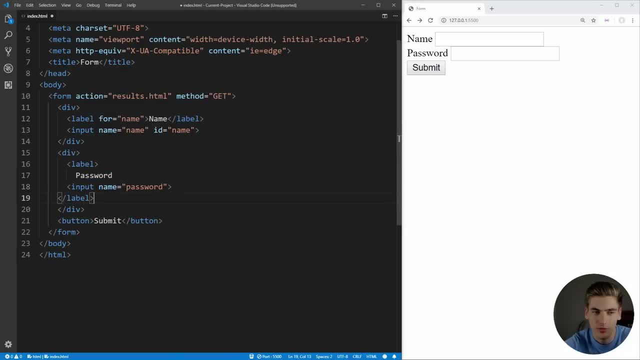 inside the label. So if we come in here and we wrap our label around our input element, so we have both our password string and our input element inside of the label. Now when we click the label, you see it's going to highlight that password field for us. Almost always, you're. 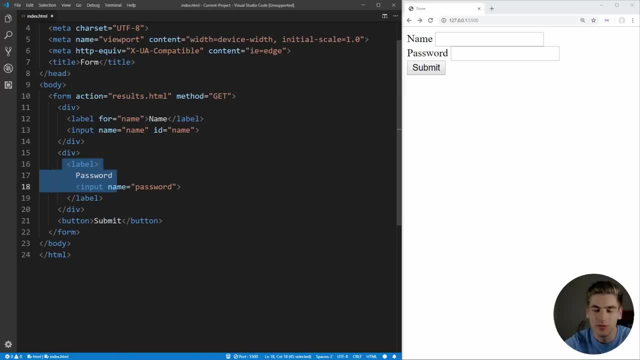 going to see people use the for attribute instead of wrapping inside of it, just because it's cleaner and easier to style. But just so you know that you can do this and a lot of people do this when it comes to checkboxes and radio buttons, which we're going to get to later in. 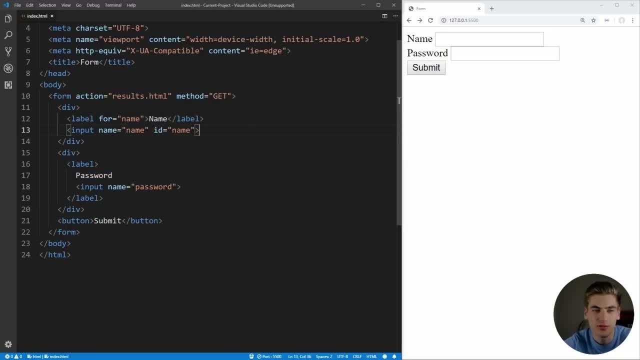 this tutorial And speaking of different type of input elements, one thing you'll notice is that our input here does not have any type specified for it, which is why it's defaulting to a text input here. But you always want to be explicit in what type of input you're using, So you always 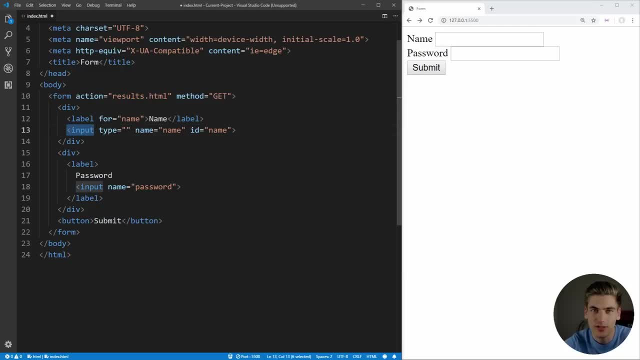 want to specify a type field And the input tag is very versatile because you can have many, many different types of inputs. But in our example we just want to have a text input here for the name But for the password. normally when you're on a website, 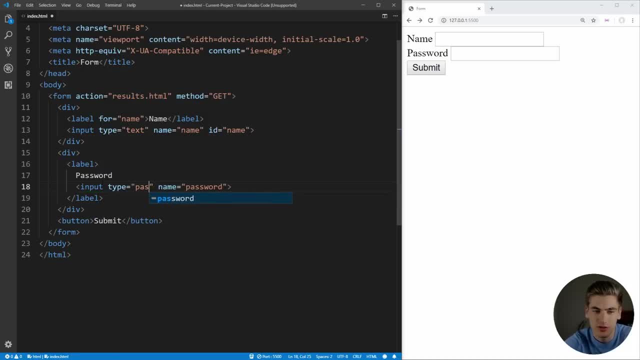 when you type in your password, it's actually hidden, And that's because there's a type which is called password which actually by default hides the characters for you. So now, if we save this and we enter our username, you see it works just fine. But when we enter a 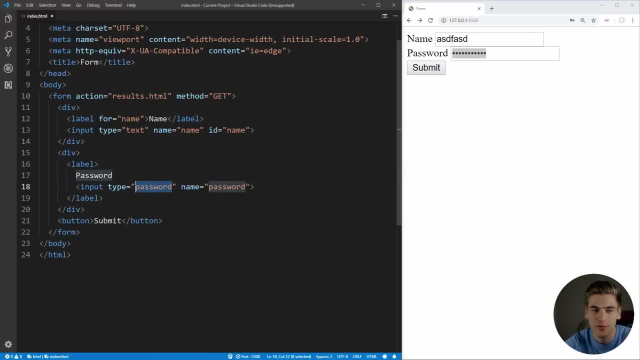 password. you see, it's hiding our characters for us And that's because we're using type of password for our input element. And lastly, the only thing left to make this login form correct is that we need to change our button down here, because we want this to be a submit button, So we can just 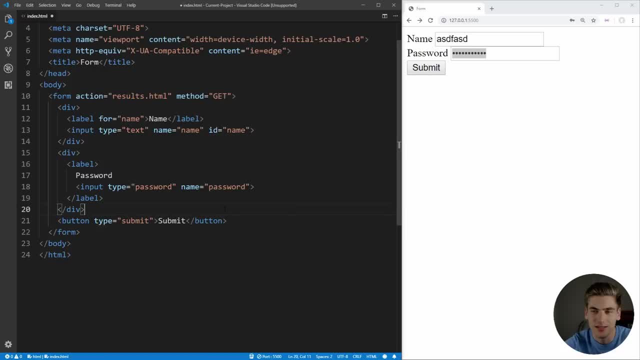 come in here and we can type in the type of submit And what this says is: this says it's going to submit our form And when we hit enter, for example, anywhere in our form. So if I type in something here and I click the enter key, it's also going to submit our form, which? 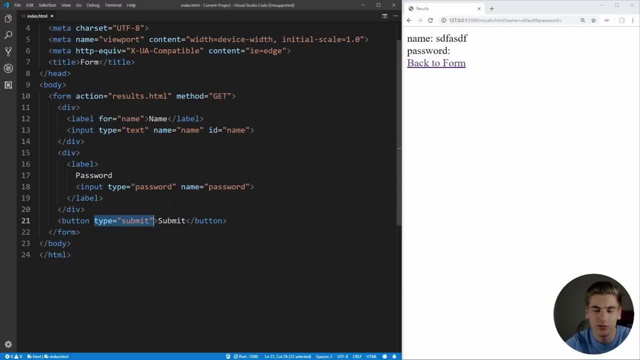 is why having type submit on your button is really useful And it also allows you to have other buttons in your form that don't necessarily submit your form, because this one right here is submitting it, since it has the type of submit, Another type of button. that's really useful and 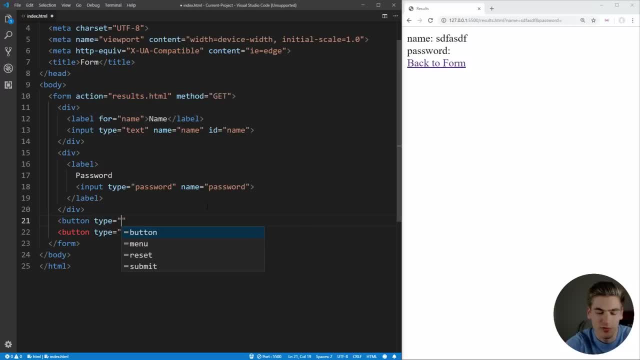 really under known is going to be a button with a type of reset. And if we just set that here, we're just going to set the text here to reset And we go back to our form. And we're going to our form And we just type in some text. If we click reset, it sets everything back to its 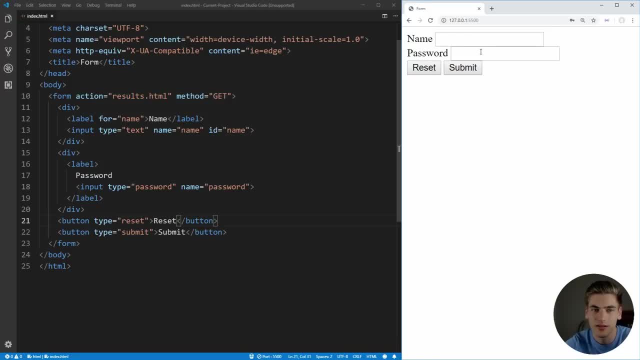 defaults And, as you can see, our defaults for us are just going to be completely blank. But what happens if, for example, you want to default the field for the user? let's say you already know what the username is for that user And you want to set that by default. That's where the value 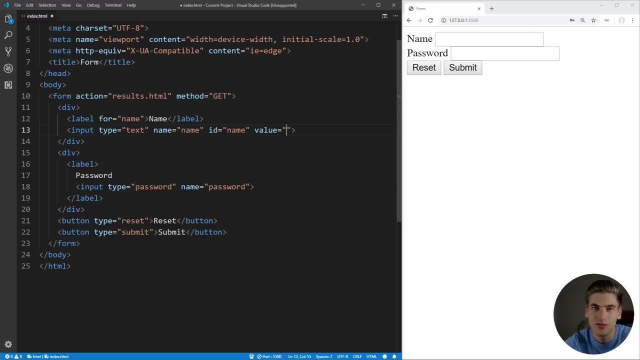 property is going to come in. So you just type in value And anything you set in here is going to be the default value for that property. So let's set the default here to just be user. Now, when we refresh our page, you see that user is going to be the default value for that property. So let's 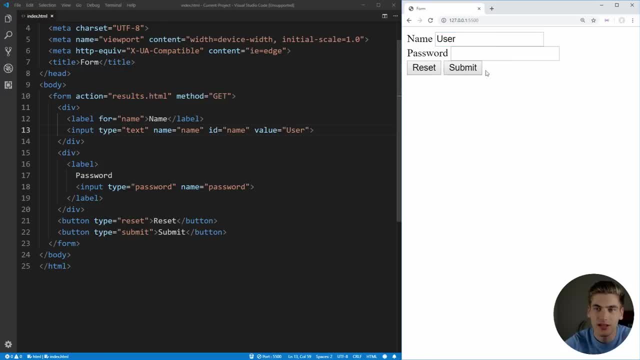 be the defaulted name, And the best part is is, if we change this and click reset, it goes back to the default value we have set in our code for the HTML. Another thing that's really useful is to have a placeholder value, For example, if we have this user's name here, let's say that we don't. 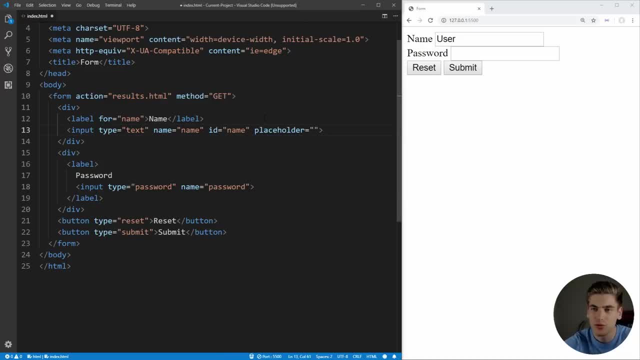 actually know what their name is, but we want to put in a placeholder. This is just something that's going to show up to kind of let the user know a little bit more information about what they want to put in here. So we're going to say our placeholder is just username And, as you can see, 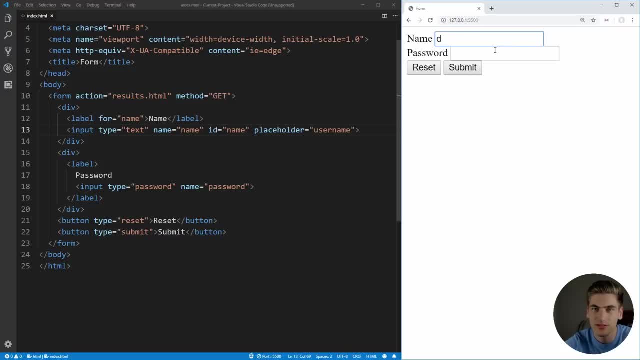 it fills that in in a lightish gray text And as soon as the user types something else it completely removes the placeholder. And if they remove everything it goes back to having that placeholder. Just to reiterate a little bit on the points that we touched on a placeholder 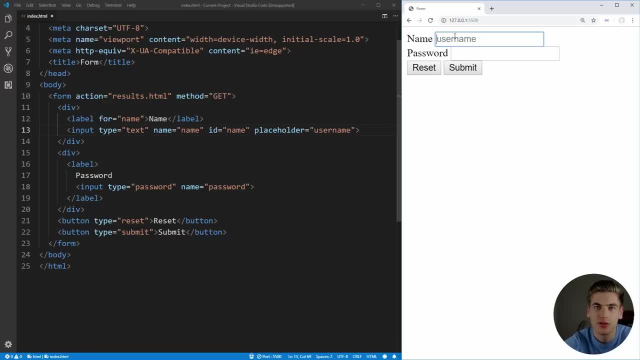 is really useful for when you want to give a little bit more information to your user while value that you set. So, for example, if we change this here to value, this is really useful if you already know what the value is or you want to default this as something that is going to be. 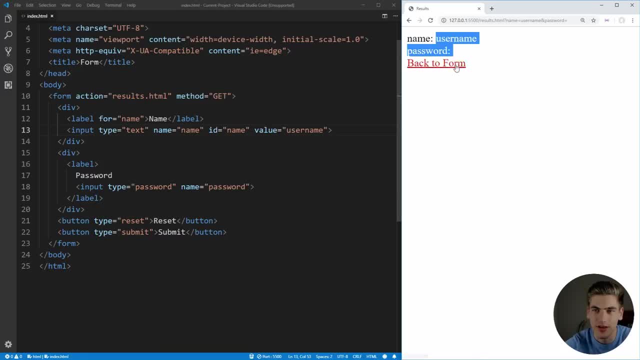 submitted with your form, Because if we click submit, it submits that username value. But if we change this to be placeholder, for example, instead, and we click submit, it doesn't not submit the placeholder, only the value. Another thing you'll notice is that we're able. 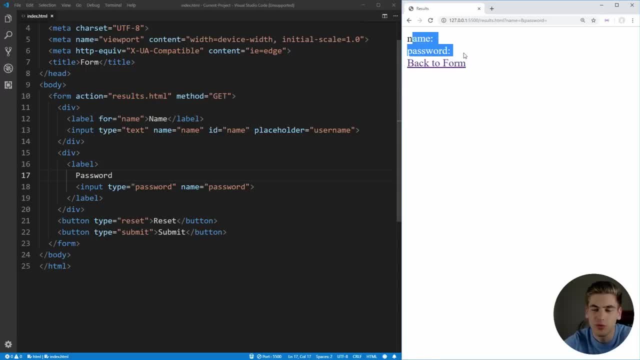 to submit a blank name and a blank password, which, in a login form, you would want to throw some kind of error to the user, telling them they can't submit blank information, And luckily this is really easy to do. There's an attribute which is called required, And this required attribute is: 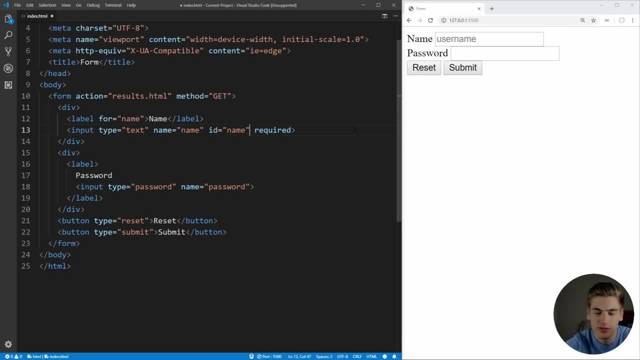 forcing the user to actually enter this information. Let's remove this placeholder So it's a little easier to see, And if we save it and click submit, you'll see that we get an error that says please fill out this field, And if we fill it out and click submit now to let it go through. So we want. 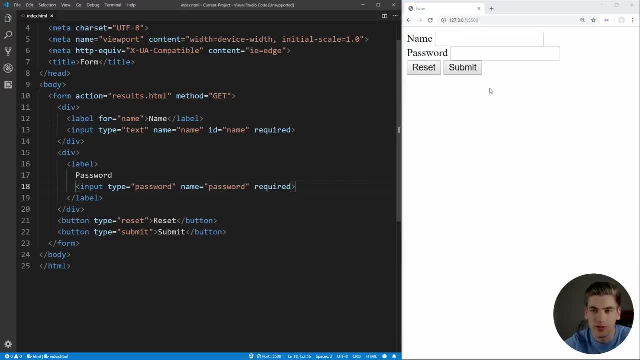 to add that required attribute to both our password and to our name field here. So now they, even if they enter just a name, no password, it's still going to give them that error until they enter that password as well. Now, as I mentioned earlier in this video, the input element here has: 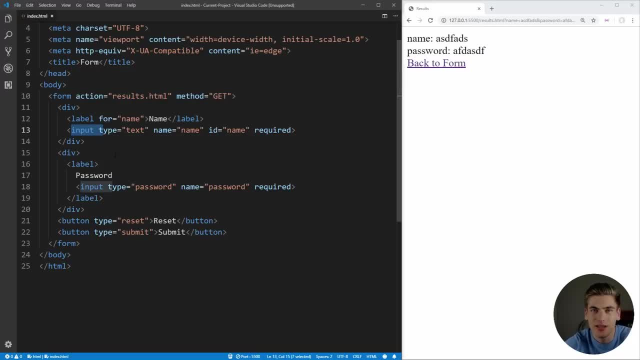 many, many different types that it can be. So let's go through and analyze some of the different types that we have, By starting with one of the most common types, which is going to be the email type. let's create another div here. this div is going to be used to ask for the email, So we're 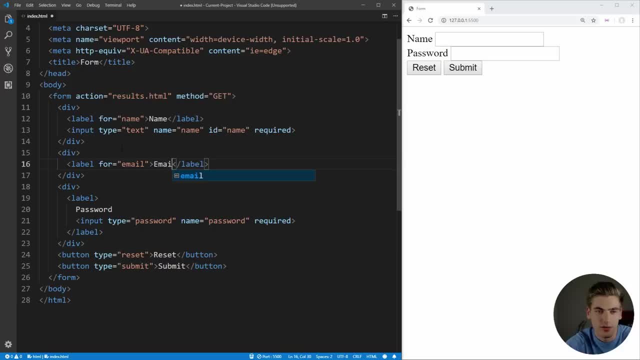 going to have a label we're going to use for email And in here we're just going to put email as the label And then we're going to create another input And this is going to have a type here of email And this is going to verify email addresses for us by default. let's make sure we 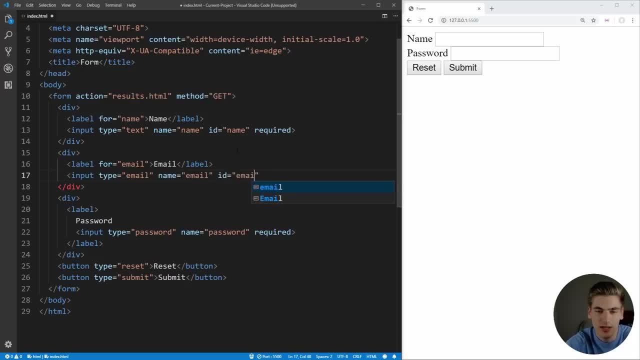 set the name to email so we can use it when we submit it, And we also need the ID here to match what we set for our four. So we're going to use email in there And let's just make it required, because we always want our user to send an email. Now, if we say that, you see, our email field is. 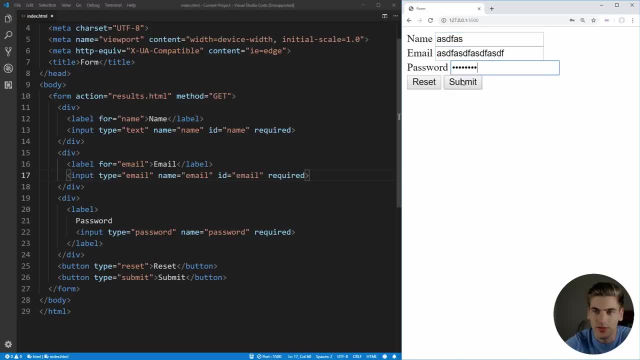 showing up here And if we type in something- for example, let's type in everything- and we click submit, you see that it says to please actually make sure that this is a valid email address. so by default, our browser is doing email validation for us. Now, it's not the greatest. 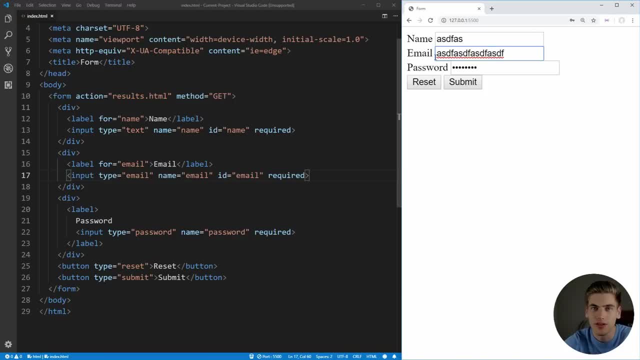 email validation in the entire world, But it's a whole lot better than having nothing, And also, when a user is on a phone, it's going to give them a keyboard which is actually specified for entering emails, as opposed to just the generic text keyboard. Other than that, though, email is. 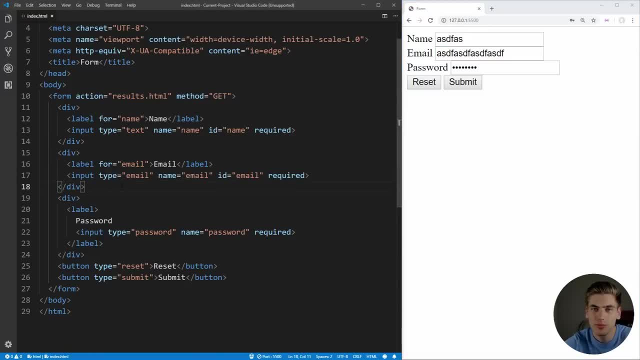 very similar to the text field that we've already covered. Now let's move on to a little bit more complicated of a field, which is the number field. So let's again enter another div in here with the label: this is going to be for what we're going to put as our age, because we want to. 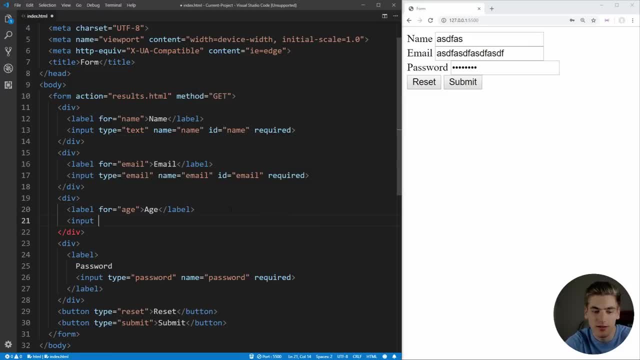 ask the user for their age And we're going to create an input again for doing that And this is going to have a type here of number And let's make sure we set a name which is going to say age and an ID which is going to be age And let's just not make this one required because we don't. 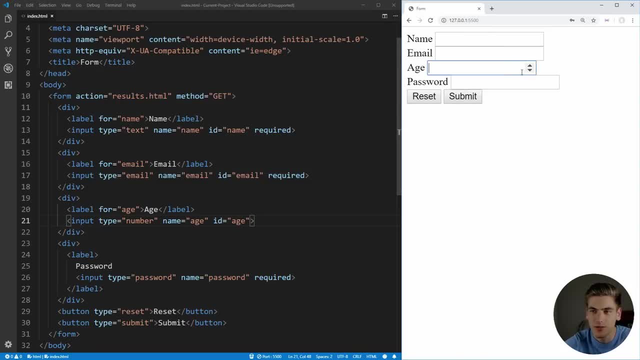 think that they need to enter this And if we save, you see, we get age And immediately you'll notice. we have up and down arrows to be able to specify where our age is going, as well as we can use the arrow keys to modify this, And that's because we're using the type of number when we 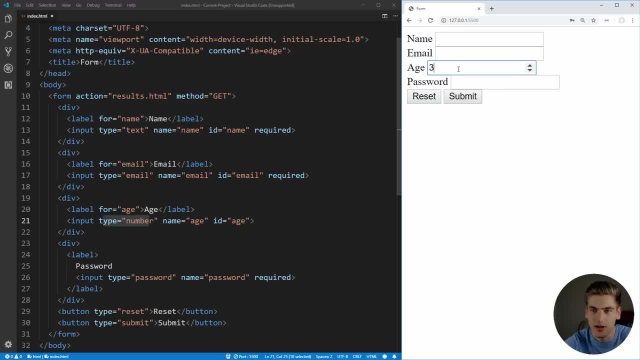 specify this input. Also, if I try to enter different characters that are not the same- not numbers- it won't allow me to enter them. Another really useful thing that we can do when specifying number elements is we can specify minimum and maximums. So obviously we don't. 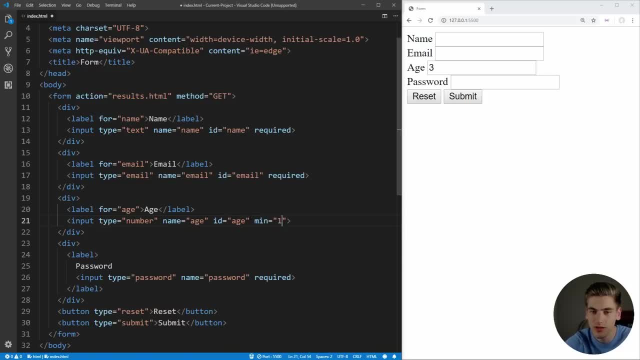 want our age to be below zero, So we're going to set the minimum here to be one, And we also don't want it to be above a certain number, So we're going to set the maximum to just say 200.. No one's. 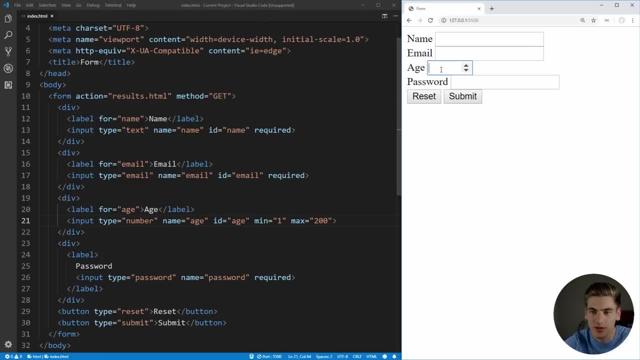 over 200 years old. So now, if we save that and come over here and we try to decrease this, you see that one is the lowest we can go. If, for example, I enter negative 10, make sure all the required fields are entered and hit submit. Oh, let's make sure this is. 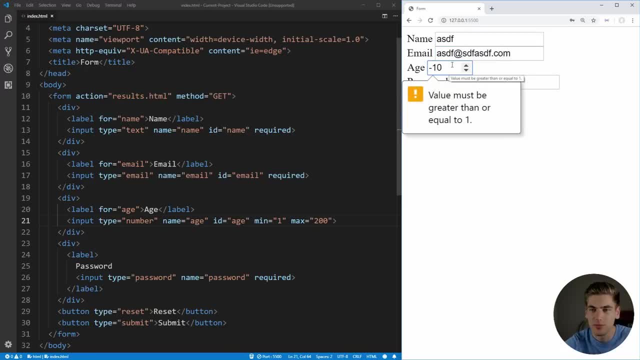 actually an email, And now we click Submit, you'll see that it says the value must be greater than 10.. But let's say we put 201 in here, click Submit, you'll see that it must be less than 200.. So these: 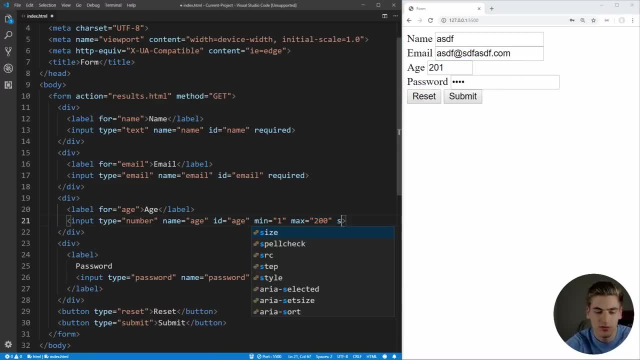 validations are built into the browser. Another interesting thing we can do is what's called step, And by default the step is going to be equal to one. So that means when we click our up and down arrow keys it's going to increase and decrease by one. But, for example, we could change this: what? 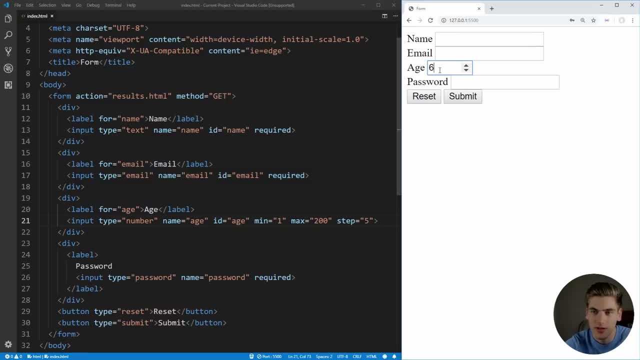 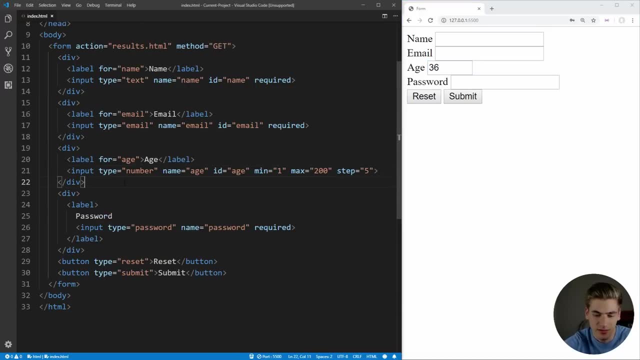 if we wanted it to be by five. So if we save this now, when I click up, it's going to increase by five at a time. as you can see, The next input element we want to cover is going to be the date input element, And again, this is going to be just. 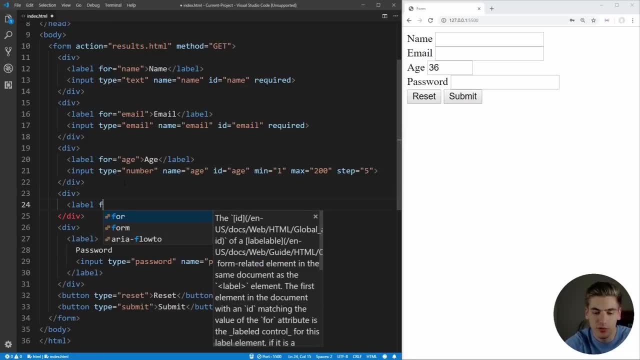 like all of our other input elements, we're going to have a label which we're going to set a four to. in our case we're going to say for date, And we're just going to come in here and we're going. 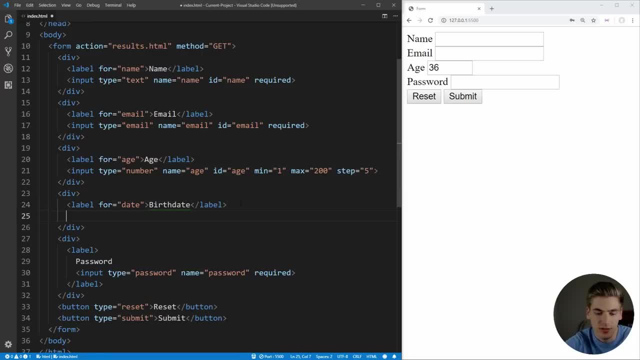 to say this is going to be a birth date, for example. So now let's go down here. we're going to create an input And this is going to have a type, And we just want to set this to date, to specify to date. we're going to make sure we set the name to date, the ID to date, so that we match our four. 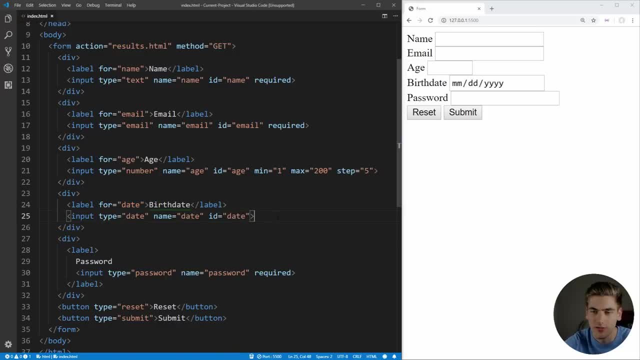 for our label over here And we're just going to close that off. And now, if we save, you see that we get a date input which already has some defaults for us, as well as a nice little date picker where we can select what date we want inside of here, just like with the number field. 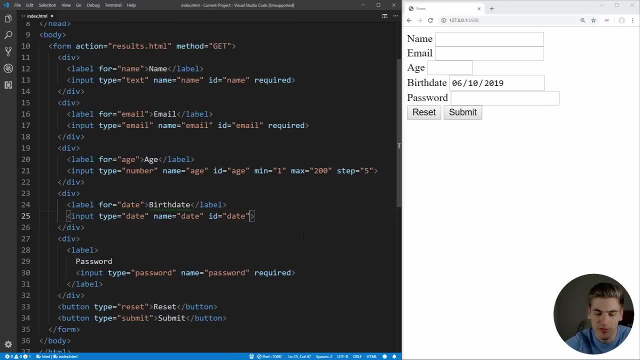 we can, for example, specify a minimum and a maximum if we want. So let's come in here and specify a minimum, which is just going to be 2019.. June 10, let's save that and come in here. And if 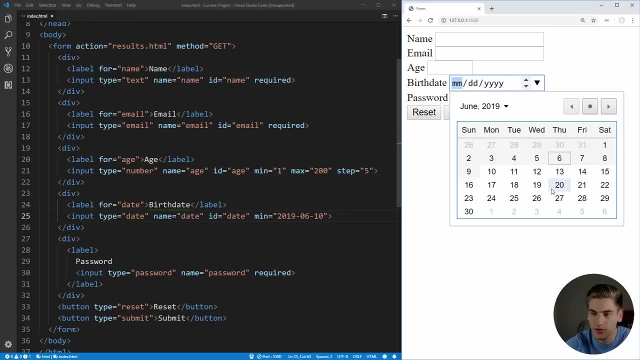 I try to select the date before that. it won't let me, but it will allow me to select the day after that. And if I come in here and manually change this, for example, I want to change it to the first and I tried to submit it after making sure all the other fields are selected. So I'm going. 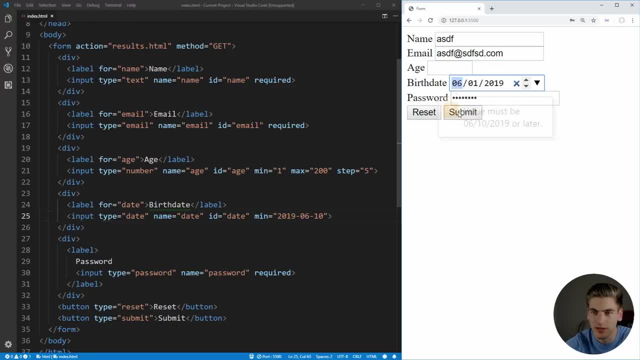 to make sure all the other fields are submitted properly. Make sure all the required ones are. click Submit And you'll see that the value must be greater than that date that I specified as the minimum. And again, we could do maximum if we want, but we already did that with numbers. So 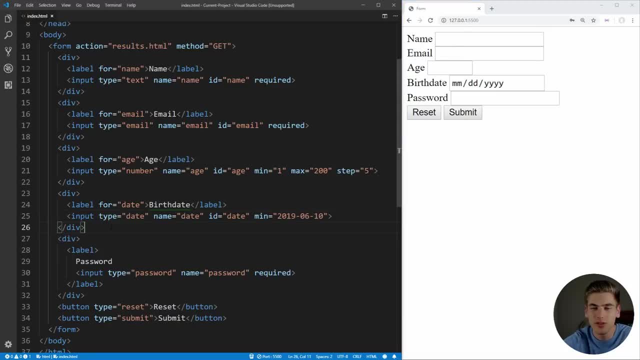 we're going to skip that. Now let's move on to the next type of input, which is going to be completely different than all the types we've covered so far. this is going to be the checkbox element. So let's create a div, And inside of this div, we're just going to specify a little. 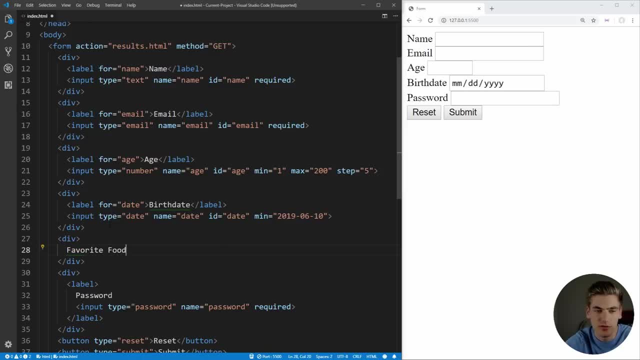 bit of text. this is going to be outside of a label And this is just going to be for favorite food, because we want checkboxes for all of our different favorite foods And now inside of here we're going to put all of our different checkboxes, we're going to do each. 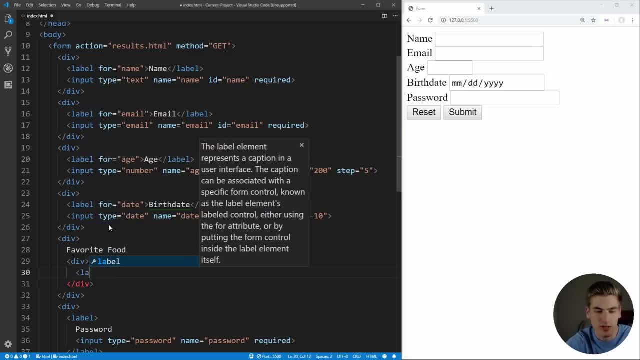 one of these inside of their own div. So, firstly, we're going to have a label, which we need for all of our different elements. we're gonna have a four And this first option that we want to have is going to be banana. make sure we close that off, put in banana here, And then we actually 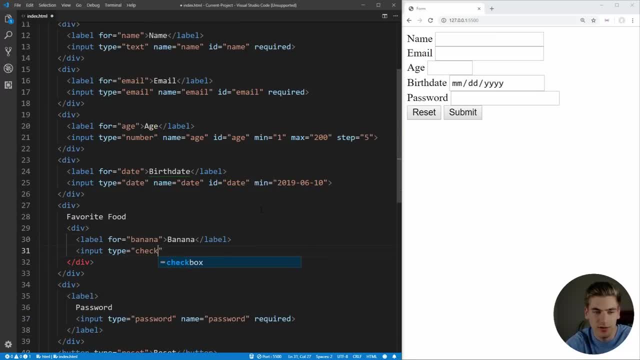 want to create the input for that. So this input is going to be a type here of checkbox. we're going to specify here our name, which is just going to be banana, And we're going to specify, lastly, the ID, which is again going to be banana. 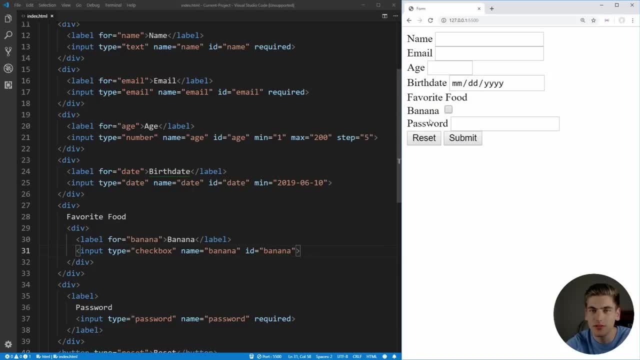 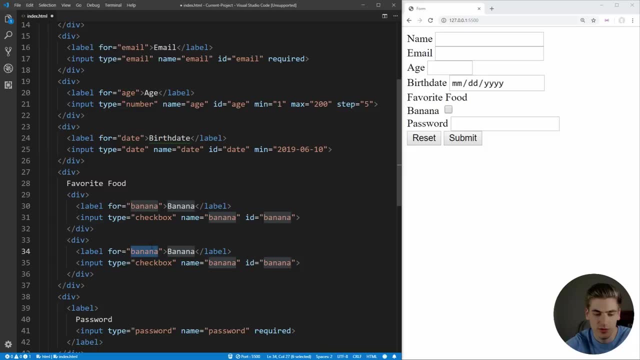 and we're going to close that off and save it. And you see, we get a checkbox here for banana. Now let's say we want to add another favorite food. Let's just copy this div so that we can do the exact same thing, But we just want to change this. So we're going to change this to be Apple. 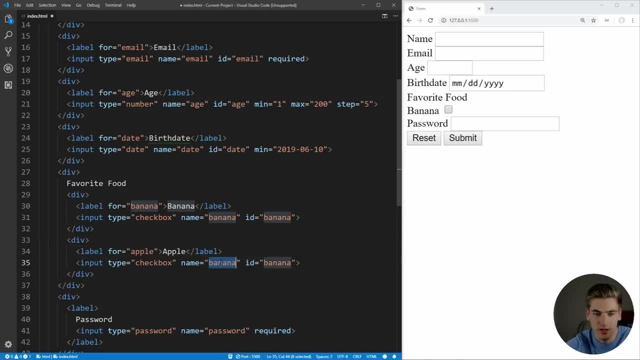 change the text to be Apple, if I can spell properly, and make sure of course we update our name and our ID to be properly set. Now if we say that you see that we have banana and apple and we can checkbox both of this if we want, or just one or none of them. But what if we only? 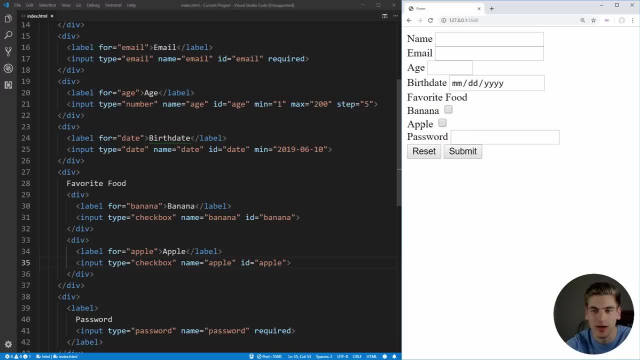 want to be able to allow a user to check one box at a time instead of all of the boxes, because with checkboxes you can check as many or as little of the boxes as you want, But if you want to allow them only to specify one favorite food, 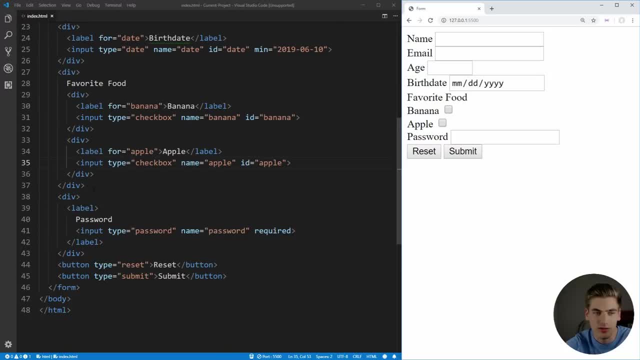 we need to use what's called a radio button. So let's go down here And we're going to create another div And inside this one we're going to ask the user for gender, because they can only have one gender, And we're going to use a radio button for that. So let's close this off here. 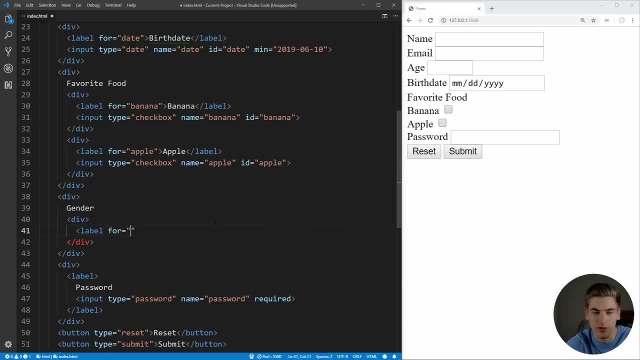 we're going to create our div, get a label inside of that And this label is going to be for our first one, which is going to be male, And we can just say male, And then we need to create our name. So the input is going to have a type here which is going to be radio, And now you would be: 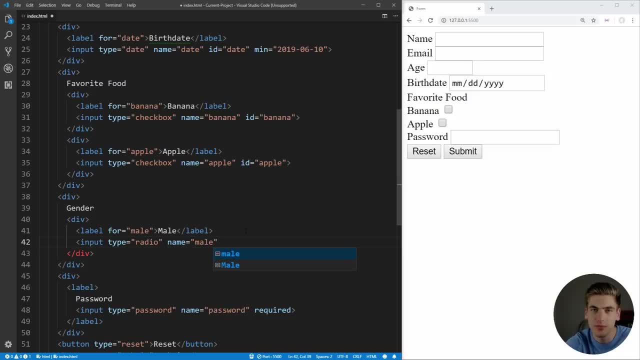 thinking that the name here should be male. That's actually incorrect, because these radio buttons all need to share the exact same name, which is how we know that there can only be one selected. So in our case, this is actually going to be gender for our name, And we want to also put in 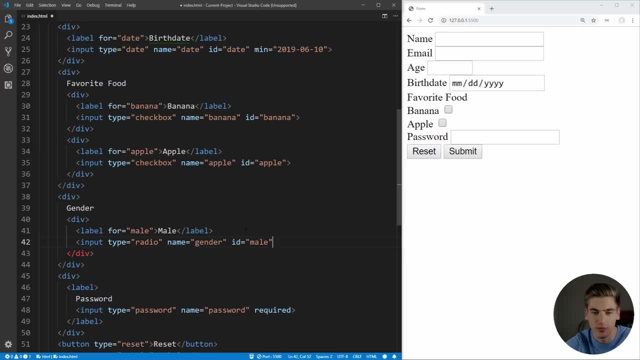 here our ID, which is male, which again corresponds with our for element for our label. Now let's save that And you see we get a radio button for male. let's add the exact same thing for female. let's copy this down. 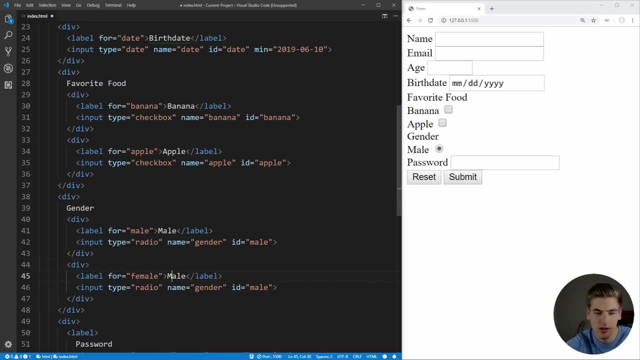 Make sure that everything's indented properly, And this is going to be female, female And, lastly, our ID is going to be female. Now, if we save that and we click male, that's all good, But if we click female, you see it unselects male and selects female for us, And that's because. 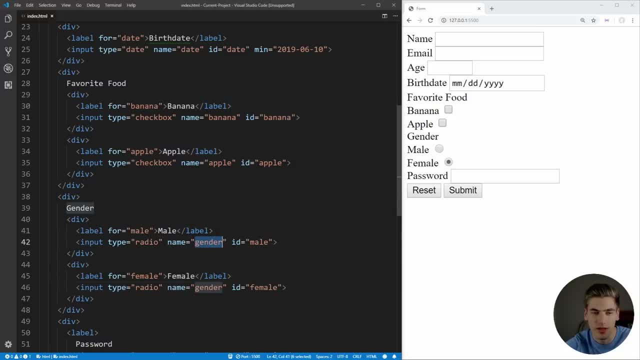 we share the exact same name of gender between both our male label and our female label inputs down here. you see, they have the exact same name, which means that we can only select one of them at a single time, as opposed to be able to select multiple of them. One thing that you need to do. 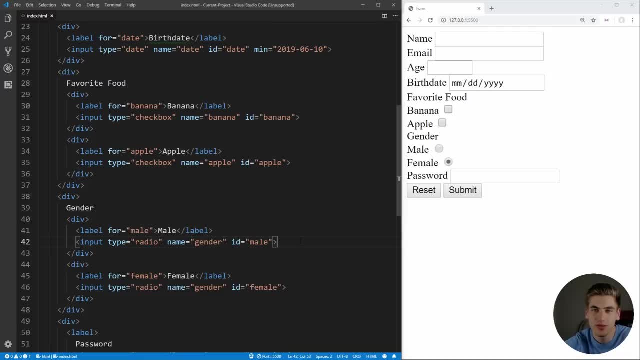 additionally with radio buttons, though, is actually specify a value, So when you submit it to your form, you know what you're getting back. So, in our case, we want to put a value here which is going to be male and for female, We want to put a value which is going to be female. 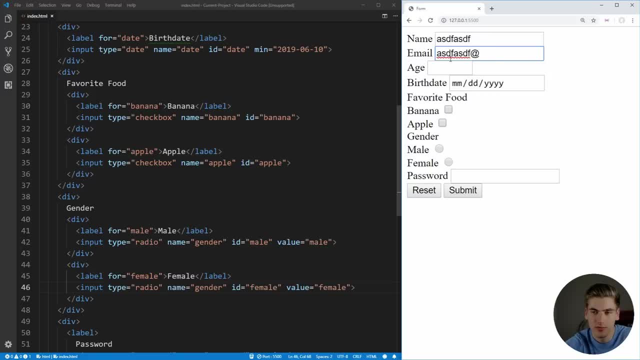 Now I'd say that and actually enter in some information for our form so that we have some valid information, And let's select male and we click submit And you'll see we get gender here set to male, which corresponds with the value that we selected here for our radio button. Now the next element that we want to look. 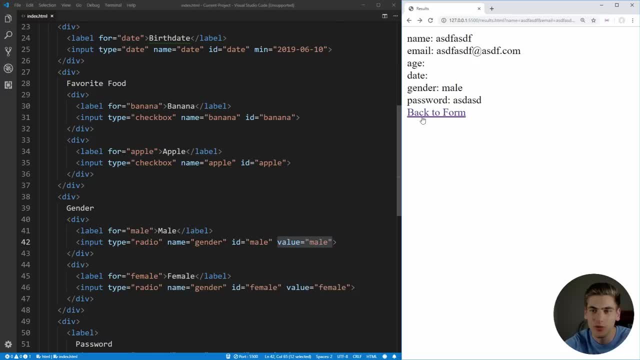 at is actually not an input of gender or fact. We want to look at the information based on decimation input element. it's actually a select element, but it works very similarly to the other input elements. let's go down here a little ways before our password and we want to come in here with our div. 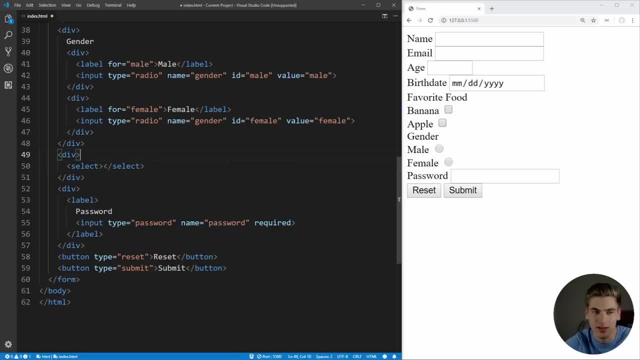 and inside of this, instead of an input, like i said, we're going to be using a select and of course, we still want to label our select. so we're going to make sure our label is specified here and inside of our select we're going to select eye color, so we can just say here, our eye color and we want our. 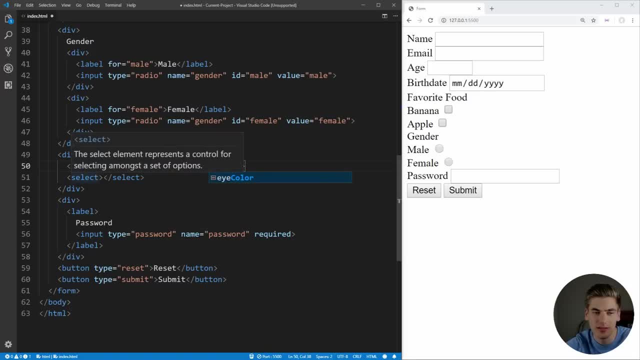 label to say that eye color, and inside of the select, what we're going to do is we're actually going to put options inside of here. so to do that, we come down here, we type in option and our option is going to have a value- whoops, a value. so in our case, we're going to put green. 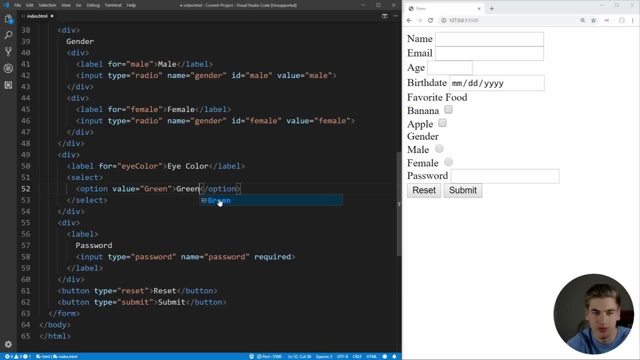 as the value and it's also going to have that in here as the actual text, so we can just put that here. you could also use what's called the label section and specify green here, so we'll do that. on another option, let's copy this down: we're going to do a red option, so we'll say red. but 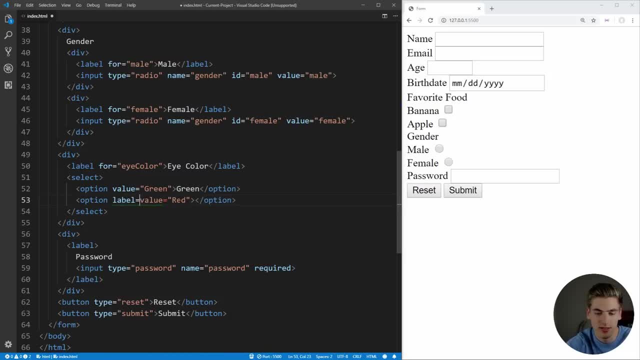 instead of putting our value inside the option like that, we'll just say: our label here is going to be red and also on our select, we need to, of course, make sure we have a name here which we're just going to set to eye color, and again our id, which is going to correspond with that label. for that, 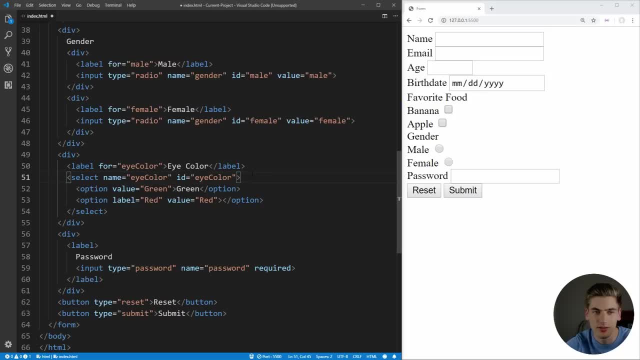 we have. so id here is going to be eye color. now let's save that and you can see, we have our eye color selector, which has green and red as our two different values that we can select from. and again, we have green specified inside the option for the label, or we can use the label attribute of our 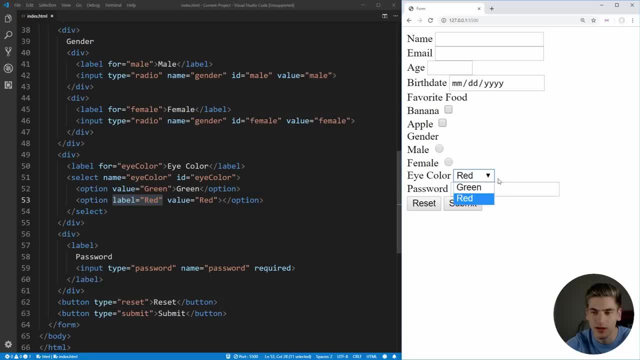 option either way, allows us to set the actual value for our label and again, we can use the attribute that we're seeing inside of the select here. now, by default, a select only allows you to select one option, but you can come in here and you can use the attribute which is called multiple. 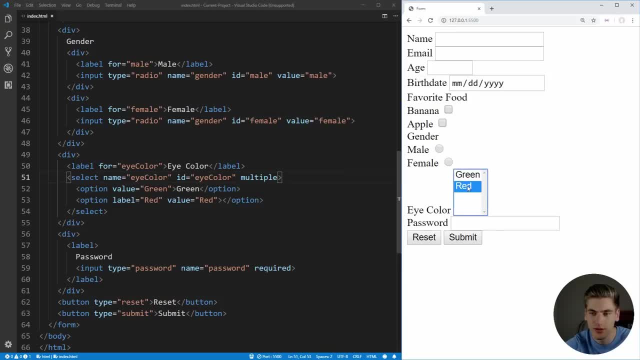 and if we say that we can now select multiple values by just holding down control and clicking on them like this, and now we have both of our values selected. and if we fill in everything else on our form, just so we can see what this looks like and mix our passwords there and we 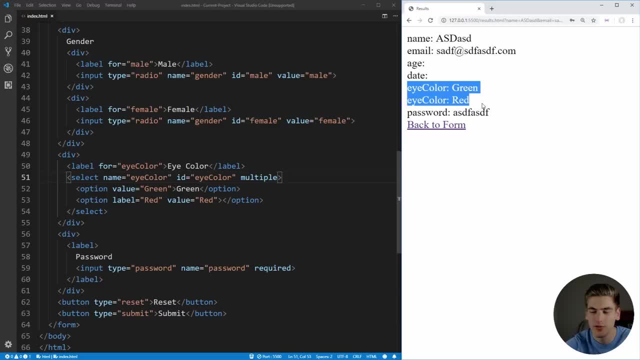 submit, you see that it has eye color showing up twice, both for green and for red, because we selected both of those values from our previous form. now, if we go back to our form and we're going to set up our text for our text and you may notice that we don't have any form elements that 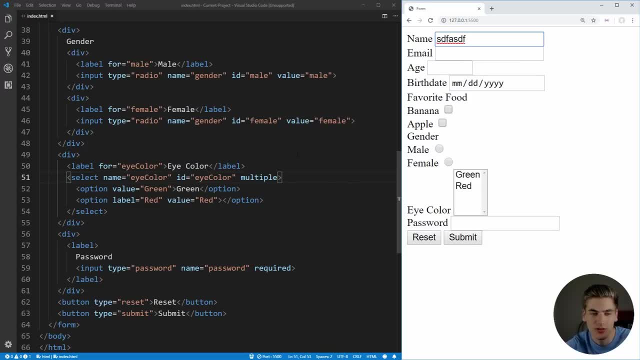 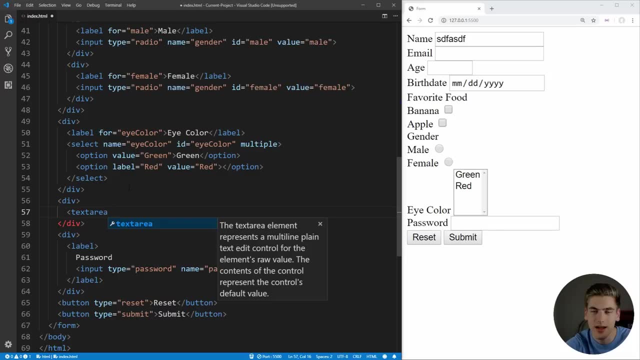 allow us to specify lots of text and text with new lines in them and etc. so in order to do that, we're going to use another element, wrap it inside of a div here, and this one is called a text area, and this, again, is not actually from an input. it's its own element called textarea, and this is one of. 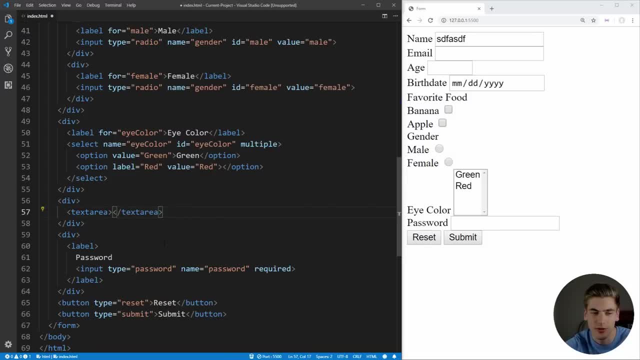 the few elements that has an actual closing tag, because the value actually goes inside of the text area here as opposed to on a value attribute. so now let's first, before we get carried away, put a label bio for our user and we could just say bio. and again we want to make sure we have an id on here. 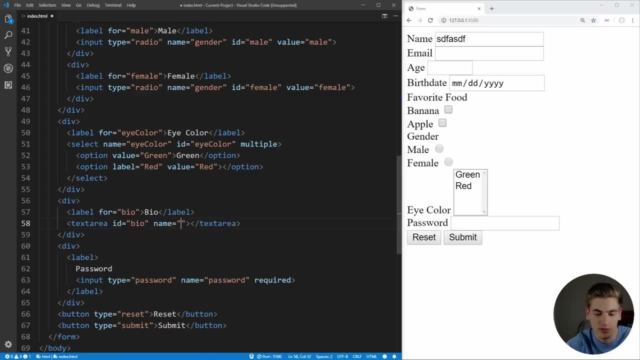 which is going to match the for from our label and a name, so we can actually use this inside of our form. and now let's put a bio inside of here. so we're going to say my name is kyle and if we save that, you see that we have a bunch of extra space being added into our element here, and that's. 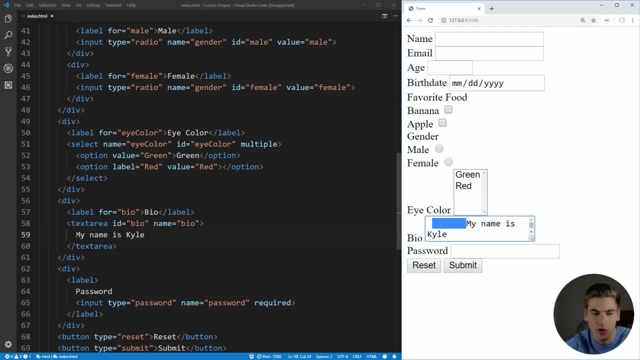 because this text area converts all of the white space. so all this white space before the my name is kyle and this new line that we have here, all that's being added in. so if you have a default value for your text area, you want to make sure there's no white space between the opening and 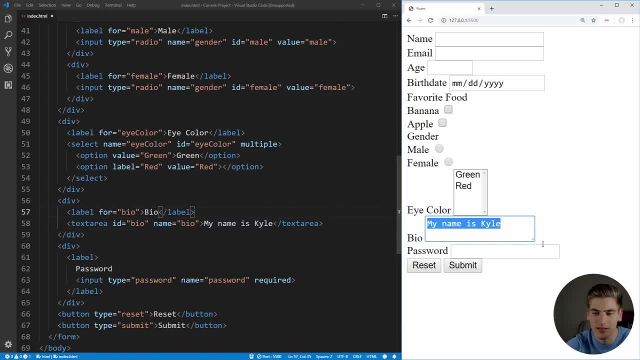 closing tags. now, if we save this, you see, that is properly not adding extra space for us, which is what we want. but let's just remove that default value for now and we save that and you see, we can enter in our value as we want. but we can also hit enter and do that and enter in multiple lines of. 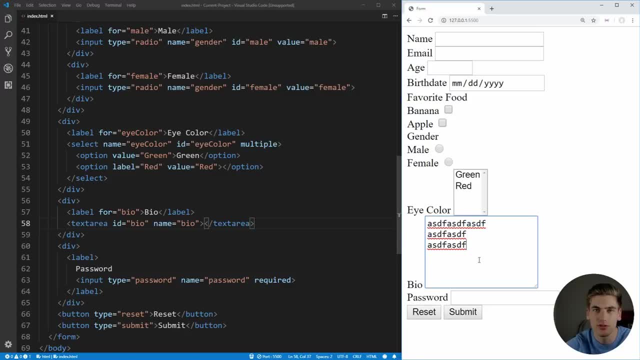 text very easily, and we can even expand this if we need to, to make it larger to work with. now, select and text area are the only two anomaly type of elements that don't actually use the input for their element. so now let's go back to the input element to talk about another really interesting element, which is called the. 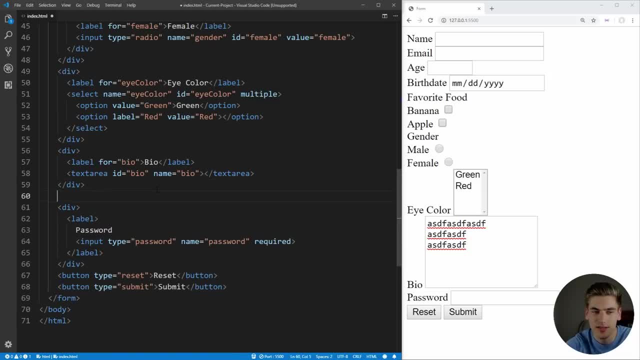 hidden input element. we don't even need to create a div for this, because it's actually just completely hidden. we won't even need a label. we just need an input and we specify the type of hidden, and that's it and we're going to give it a name. so let's just say this is going to be called. 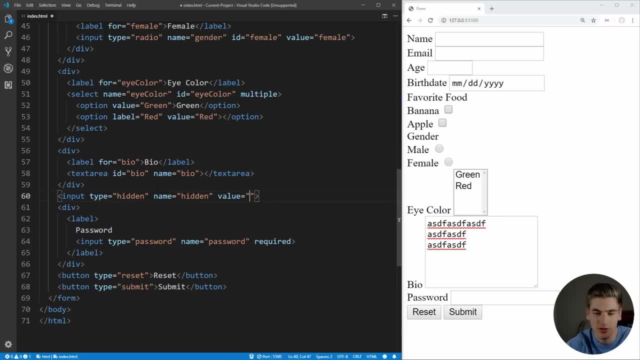 hidden and we're going to give it here a value and we're just going to set the value to high. now, if we say that, you see, nothing actually shows up on our form. but if we do submit this form, so let's make sure we submit it. 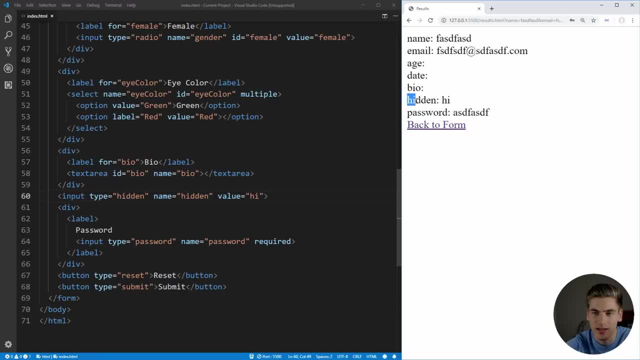 with all of our different required values and click submit. you see, we get that hidden attribute being passed along with the value we specified inside of our html, but it doesn't actually show up on our page, which is why it's a hidden input and users are not able to interact at all with. 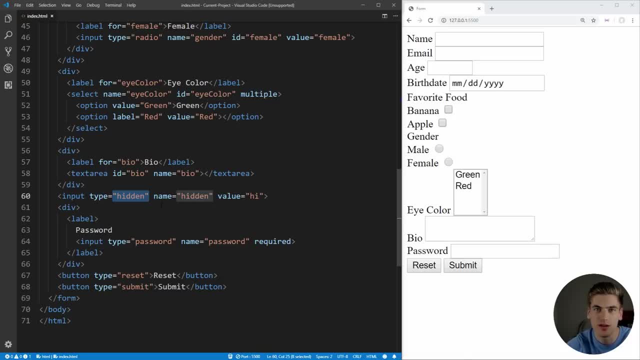 hidden inputs, which is exactly what they're used for. they're really great when you're trying to do some fancy manipulation in javascript or you want to send something down from your server. but if you're just creating a generic html form like this, the hidden attribute is almost never. 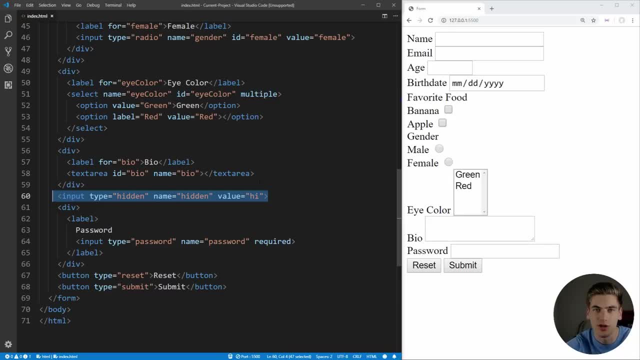 going to be useful, unless you're doing something fancy in javascript or on your server. the next interesting element that we have to take a look at is actually going to be the file input, so let's create a div so we can wrap this in here. let's create a label for it first. this is just going. 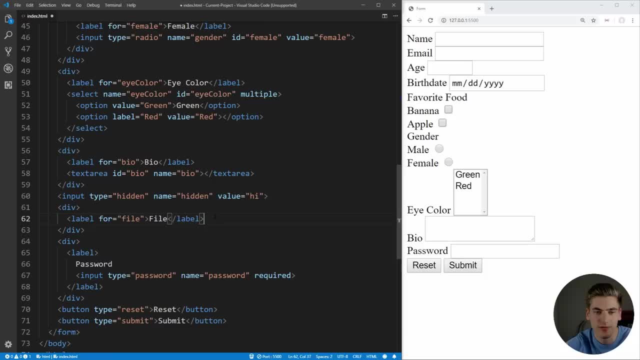 to be for what we'll just call file and we can just specify it as file. then we're going to have our input tag. we want to say that this is going to be an id of file, just so it has the same as our label. the type here is going to be the same as our label, and then we have our input tag, which. 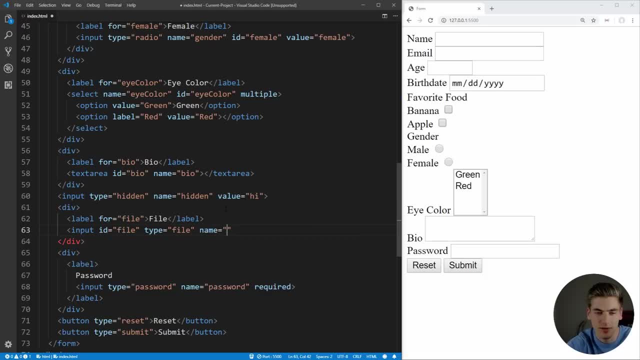 going to be a file type and again we're just going to give it a name of file so we can know what it's actually looking for when we submit our form. and now you can see down here, we can actually choose a file to submit to our browser. but the 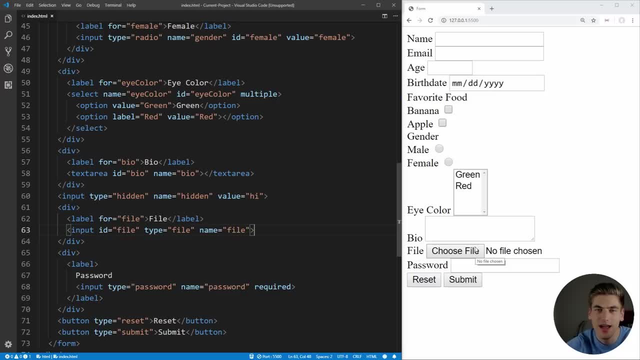 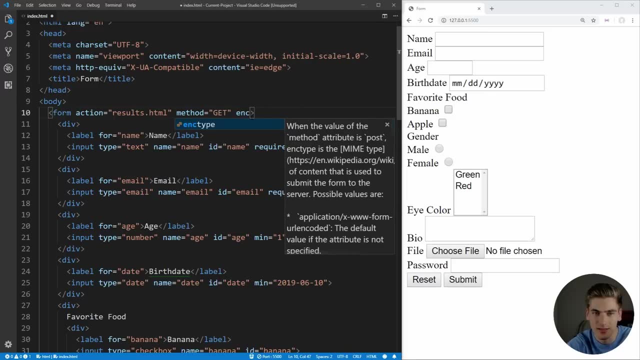 first thing we need to do to make it so that when we submit this to a server, that it's actually useful for our server. we need to specify a new attribute on our form here, and this is going to be called the ENC type, just like this, and 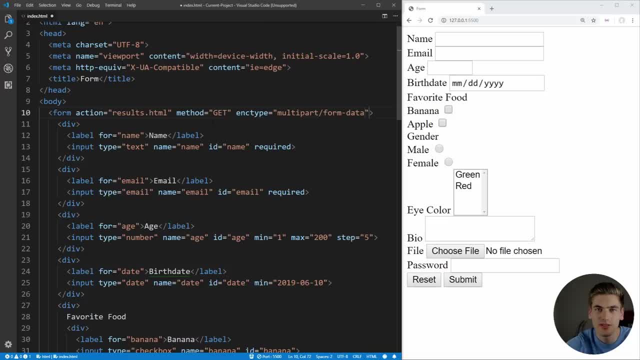 inside of here. what we want is multi-part form data, and what this essentially says is: files are very large. we can't send them all at once. it's going to send that file in multiple parts. so we need to tell our server that we're sending in multi parts our form data into multiple different sections. so 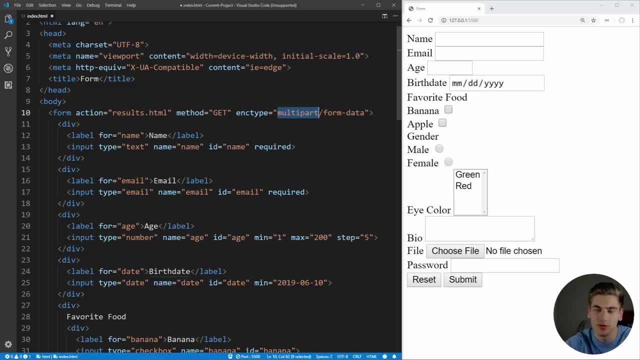 that knows, to look for multiple sections of an upload as opposed to just one single form upload, and this will actually allow us so we can submit our files to our servers. so now let's test that out. let's come in here, choose a file. we'll just choose one of my channel arts, type this in here and make sure we. 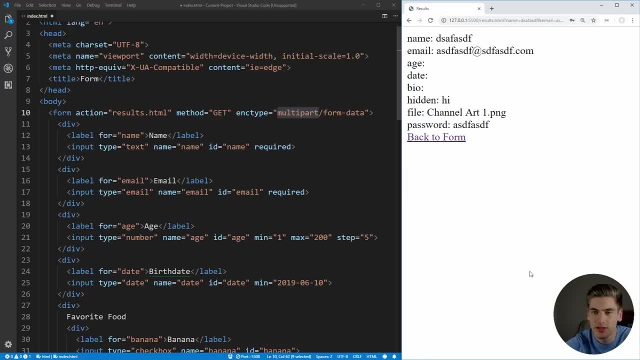 have all the different information for our form submitted and if we click submit you'll see our file is showing up as our channel art one dot PNG, which is what we selected when we uploaded our file. next let's kind of try to rapid-fire here through some of the lesser used input elements let's make sure we create. 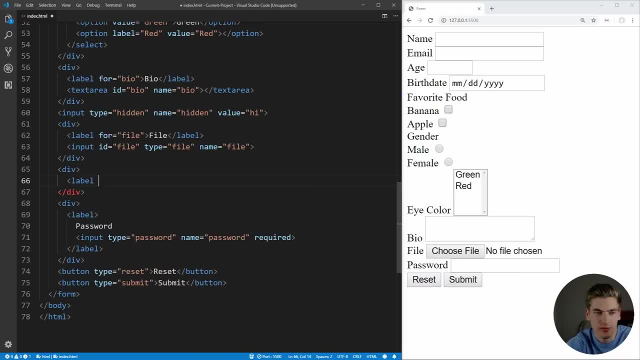 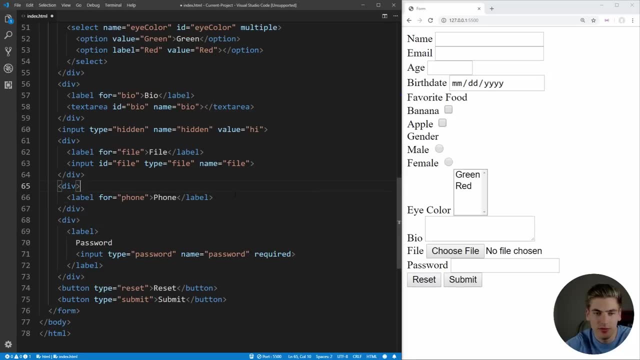 our div and inside of this div we want to make sure we have our label and this is going to be for a phone. we're gonna ask our user for their phone number, so we'll say for a phone. I'm gonna say phone is the label and we just want an. 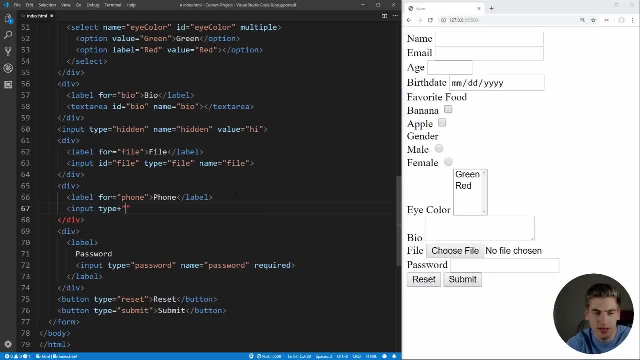 input and the actual type of this is going to be. tell TEL, just like this stands for telephone and this is going to be the type of this is going to be. name here is going to be phone whoops, phone cannot type today. this is bad phone and an ID which is going to match our four of phone. close that off and